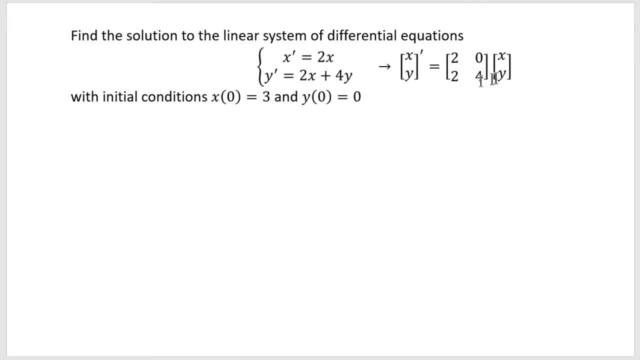 To solve this system of differential equations, first change it to a matrix form and you want to find the eigenvalues of it by writing down the eigenvalue equation. And here we see that the two solutions are 2 and 4.. Now that you have the eigenvalues, you now have to find the eigenvectors corresponding to it. So let's do lambda equals to 2, see what it gives us. That means 2 minus 2, 0,, 2,, 4.. 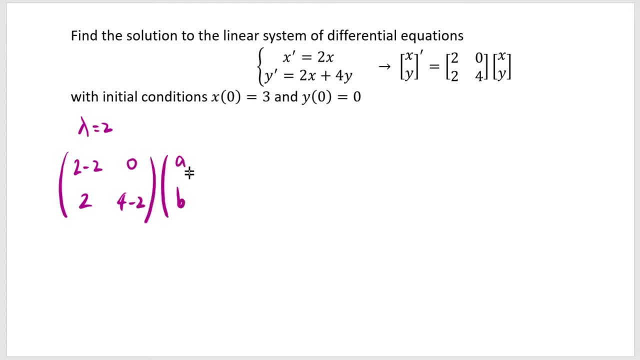 minus 2 times this eigenvector a, b has to equal to 0, 0. And this gives you 0, 0, 2, 2, a- b equals 0, 0. Which the first line just says 0,, no matter what a and b are. But the second line says 2a plus 2b has to be 0. And that means that a and b are negatives of each other And one simple. 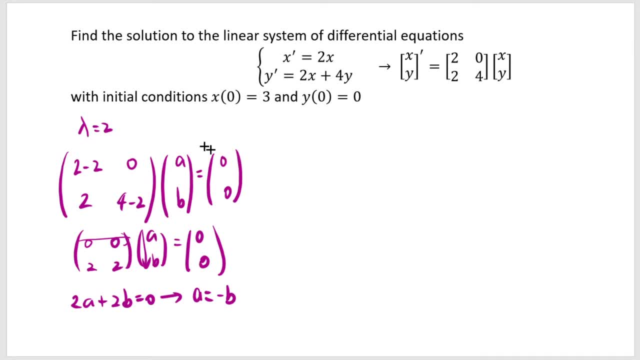 solution is just 1 and negative 1.. So we see that the eigenvector for this eigenvalue is 1 and negative 1.. Let's do another one for the other eigenvalue we found. Lambda equals to 4 gives you 2 minus 4, 0, 2, 4 minus 4 times a, b equal to 0, 0. And that gives you negative 2, 0, 2, 4.. 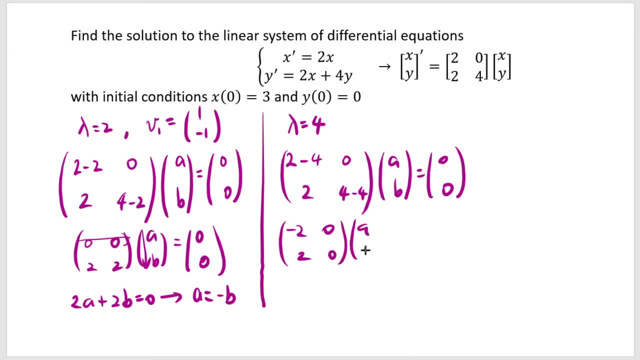 0, 2, 0, a, b equals 0, 0. And this time you just get negative: 2a plus 0b equals 0, which forces a has to be 0. And you can see that if a is 0,, regardless of the value of b, you do satisfy this eigenvector equation And for the simplest value of b, we choose b to be 1.. So we take that second eigenvector to be 0. 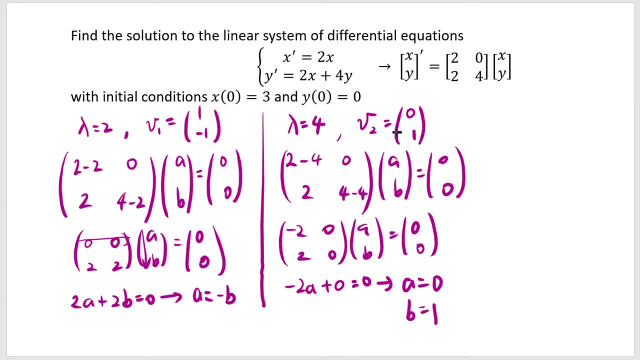 Remember, any eigenvector's multiple is again an eigenvector for the same eigenvalue. So when you solve this eigenvector equation, you have many possible solutions And your goal among them is to find the simplest one. And I found the 0, 1 to be the simplest solution to this eigenvector equation. 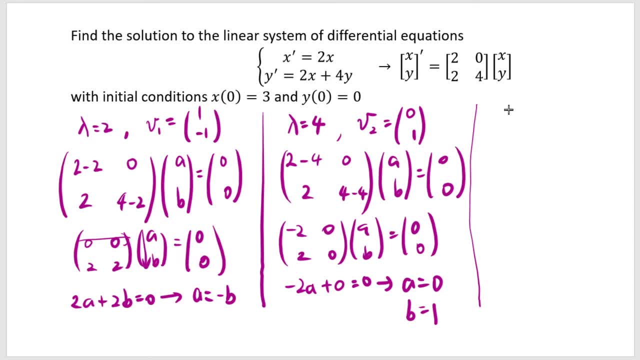 Alright, so now that we agree on that, we can write down the general solution as x, y, as c1 times the eigenvector 1, negative 1, times the eigenvector which is 2,, plus c2 times the eigenvector 0,, 1, and the eigenvalue, which is 4.. 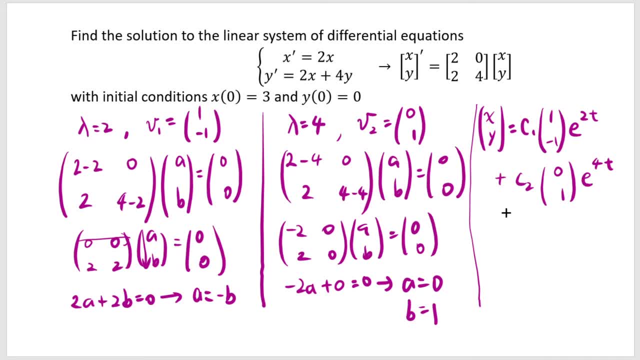 So that's the general solution. However, it's not done yet, because we need x of 0 to be 3 and y of 0 to be 0. So what does that mean? Well, if you read this solution, this really means that x is c1 times 1 times e to the 2t, and then c2 times 0 times e to the 4t. so that's nothing. 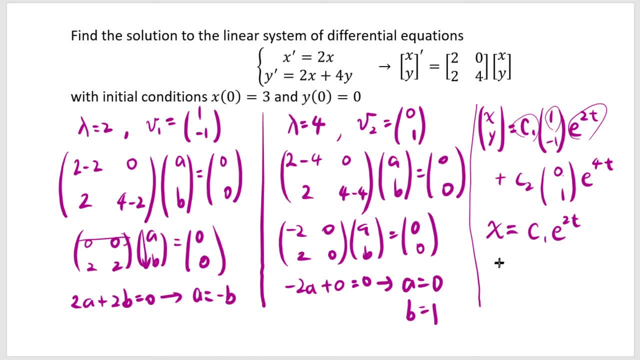 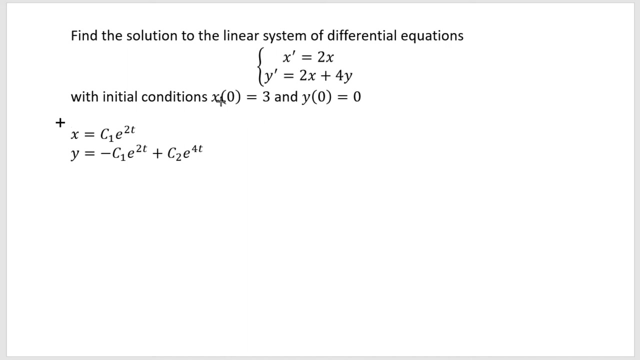 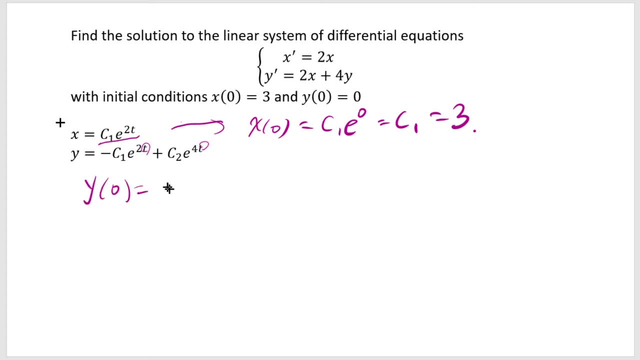 i of 0, if you plug in 0 in here, you get negative c1: e to the 0th power plus c2 times e to the 0th power, which is negative. c1 plus c2, equals to 0, that's what's requested. and because c1 is 3, we see that negative 3 plus c2 equals to 0, that gives you that c2 must be positive 3..